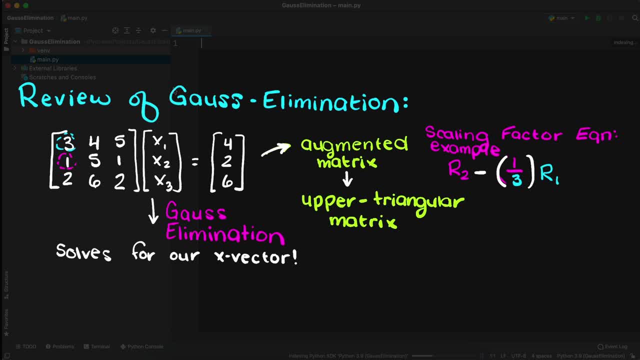 below. Then, once our matrix is in the upper triangular configuration, we perform what is called backwards substitution, which means we begin at the bottom of our matrix and solve for our unknown variables row by row, moving up our upper triangular matrix. Now that we have a broad understanding of how Gauss elimination works, let's get into 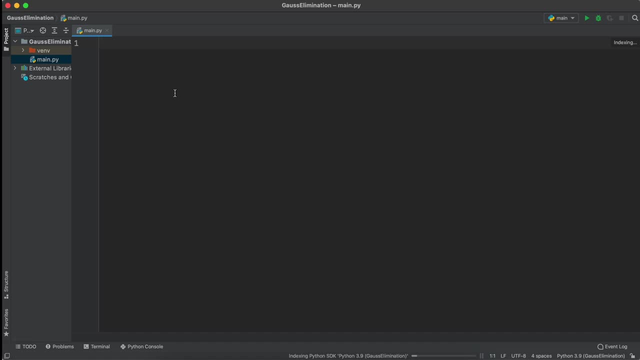 coding. Gauss elimination in Python. The first thing we need to do is import the numpy library. We are going to use the numpy library as it allows us to work with matrices within Python much easier. The IDE I am using here is called PyCharm, and to import numpy into PyCharm, I am going 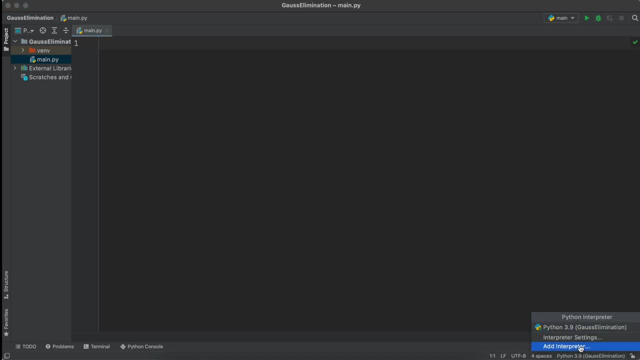 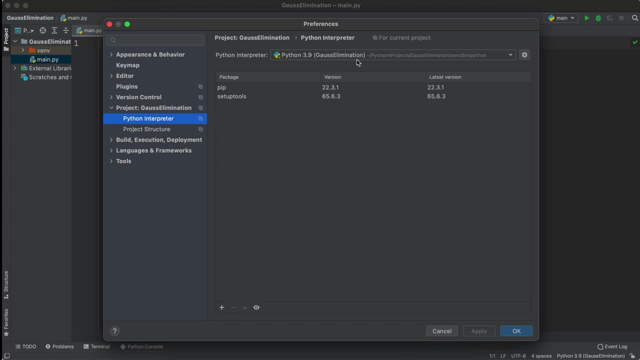 to do it in the following manner: We will click on our interpreter in the bottom right corner of our screen. Click on interpreter settings. This will bring you to the following package manager screen. Here you can find this small white plus button and click that. 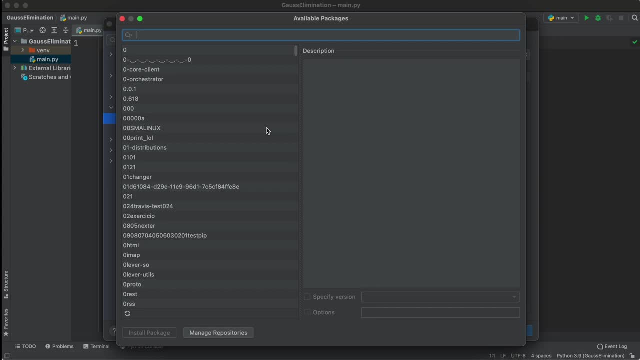 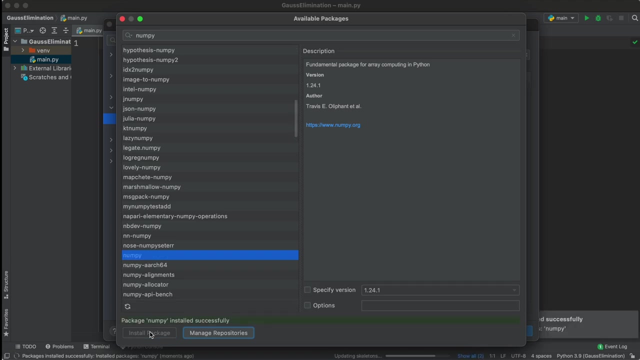 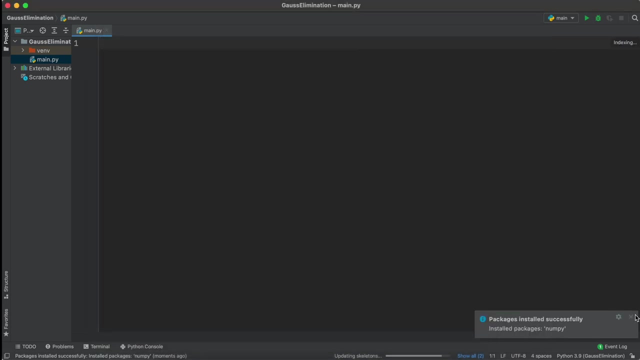 We are going to search for the numpy library and then click install package. It is very important during this stage that you install numpy to the correct interpreter, or else Python will not recognize the library when you try to run your code later in this video. 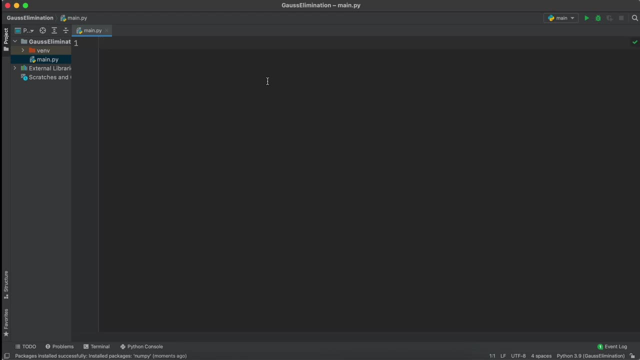 Now that all of the packages we need are installed correctly, let's begin coding our Gauss elimination. I am going to define this as a function such that it can be called with any two acceptable functions. The two function parameters that we need our user to give will be an A matrix. 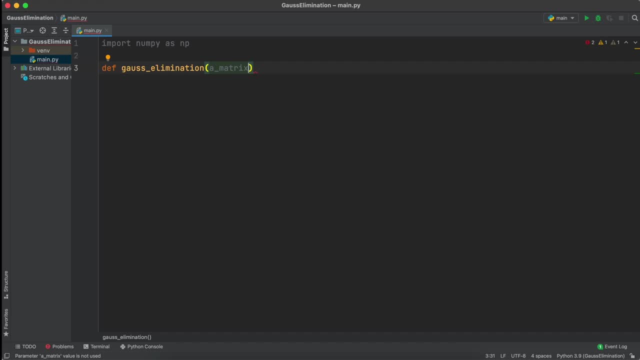 which is our linear system's coefficients, and a, B or our constant matrix. Next, I am going to add some contingencies so that our user can know if they enter something incorrectly, as opposed to just guessing. I am just going to break this up into two parts. The first 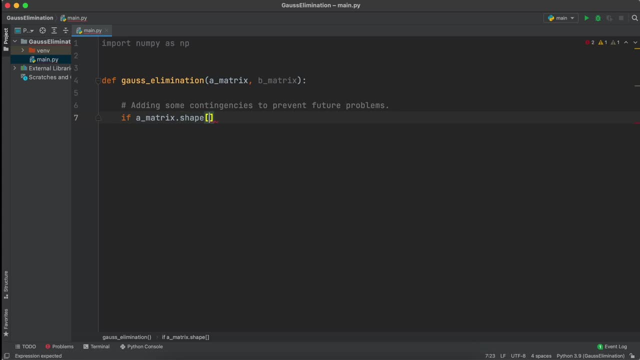 will check if our A matrix is entered correctly And the second will check if our A matrix is correct. The second part will ensure that our B matrix works with our A matrix and also that it is sized correctly. Our first contingency will use the shape attribute, which will allow us 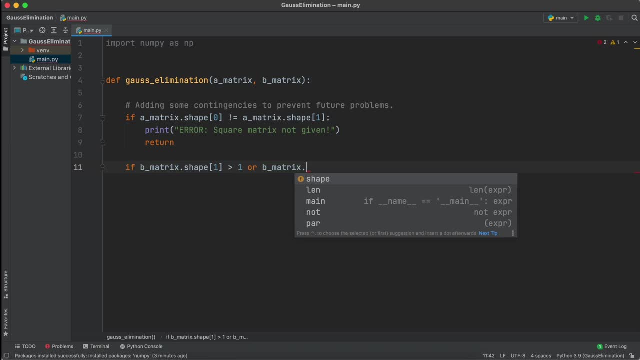 to get the row and column dimensions of our arrays. So we will first check if our A matrix that we are given is a square, as it should be. If it is not, we will return an error to our user and let them know that they made a mistake. 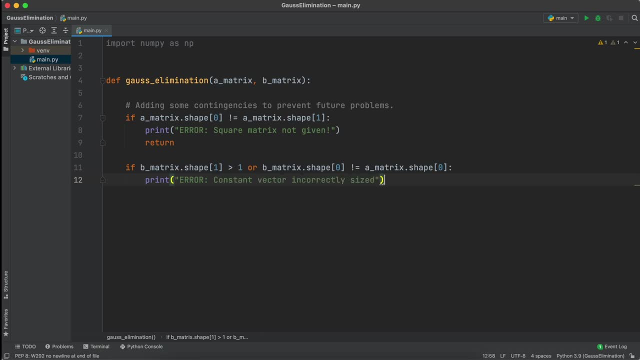 And as this will cause problems in the near future, we are just going to put a return here. This will tell Python to return to the portion of code where this gauss elimination function was called, as we don't want Python to continue the algorithm if our matrices are incorrectly. 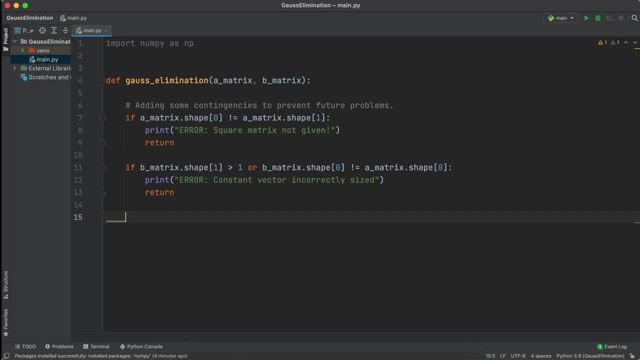 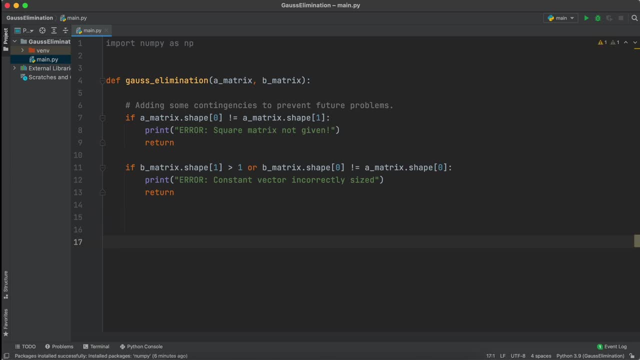 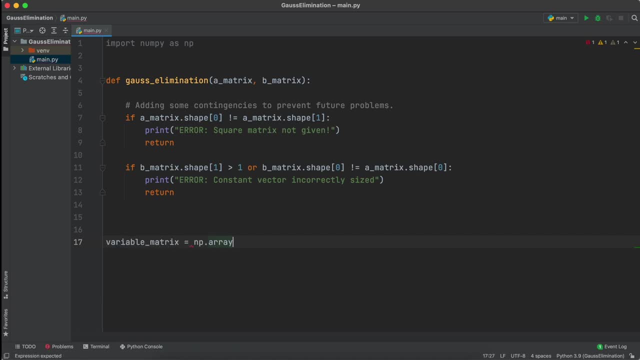 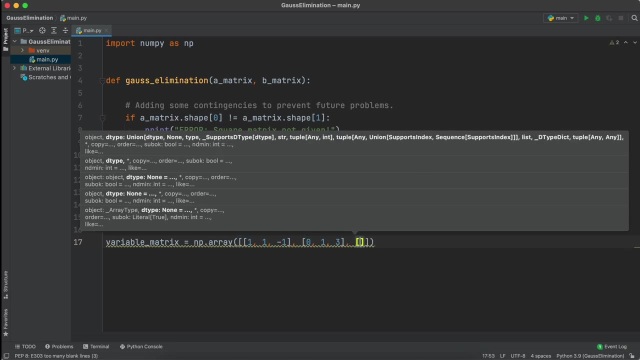 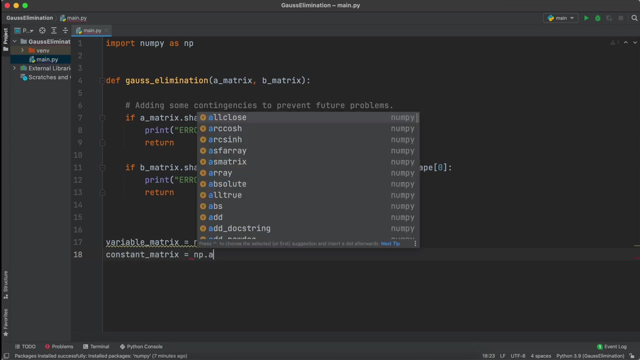 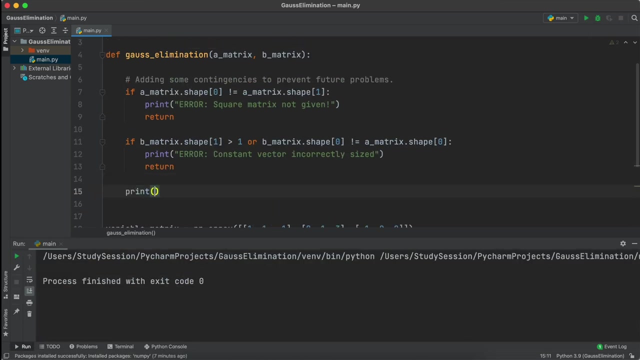 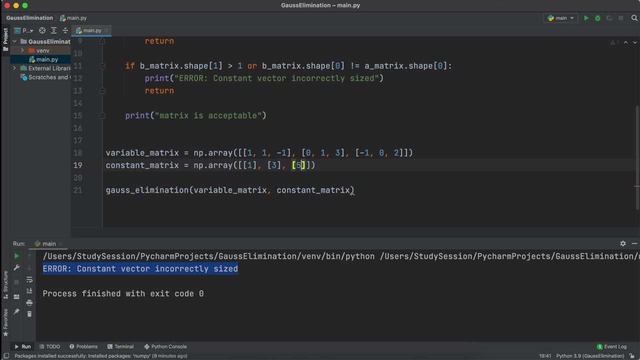 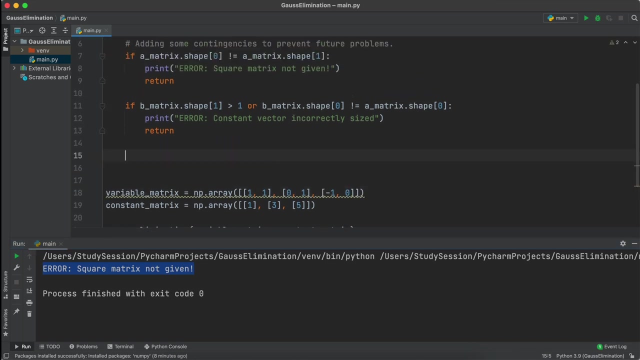 I am just going to head and enter a few matrices here to demonstrate that only a proper matrix shape proceeds through to our temporary print statement statement here. Moving forward, let's add a few lines to initialize some necessary variables. Firstly, we are going to take the length of our B matrix, which is the same as the column. 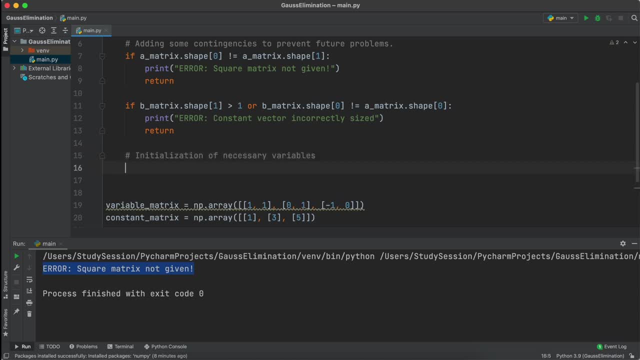 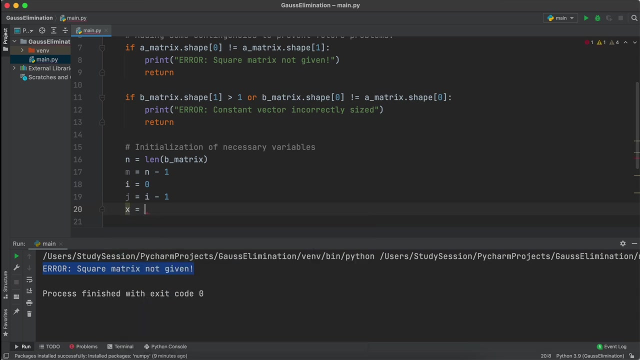 shape attribute we used earlier. Let's add in a variable that is less than 1 for our length, and I am going to add in a couple iteration variables that we will use soon. Then I will just initialize our solution vector, our x vector, using our zeroes function. 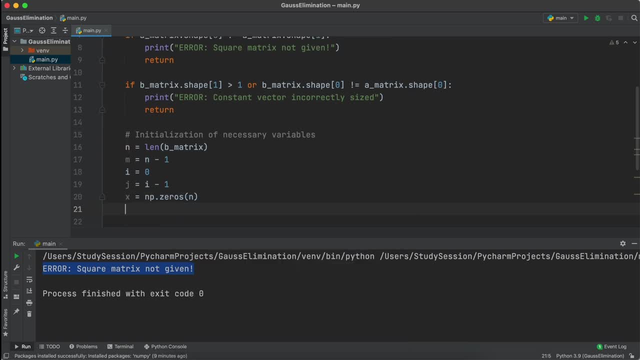 of size, n rows and one column. Lastly, I am just going to make a string variable that we will call later in our function. that will just be used for some print statements. Next, let's just complete the first step of Gauss elimination, which is creating our 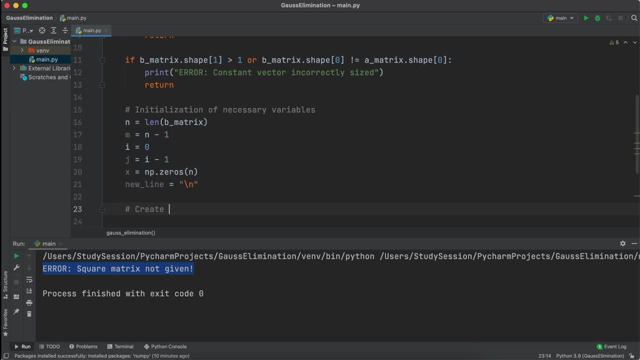 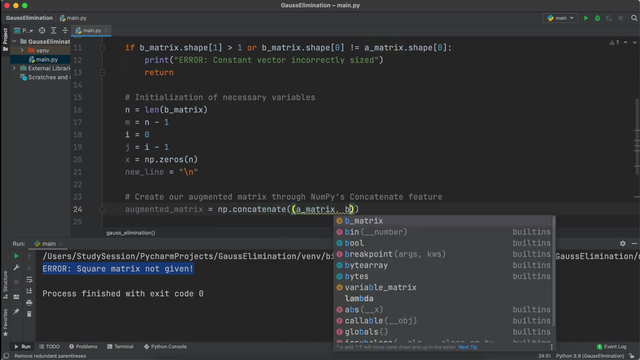 augmented matrix. I am going to do this through creating a new matrix that concatenates or adds our B matrix onto our A matrix and creates a new matrix called augmented matrix. This will be done through numpy's concatenate function, So we call our two matrices and then tell it that we want to add the B matrix in the 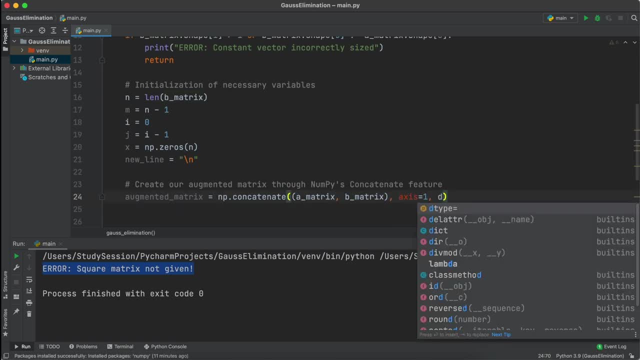 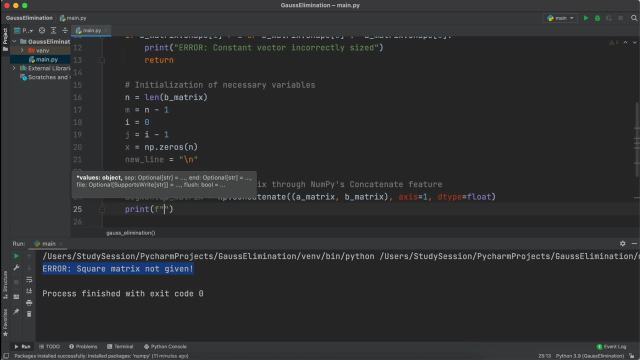 column direction, hence axis 1, to our A matrix. Lastly, I am just going to make this matrix a float data type as an integer only matrix. I am also going to add these two print statements here to show our user our beginning augmented. 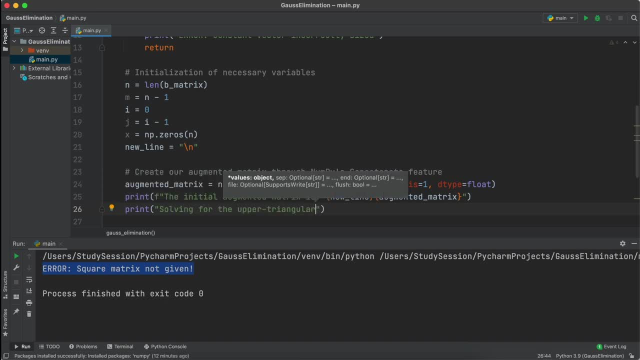 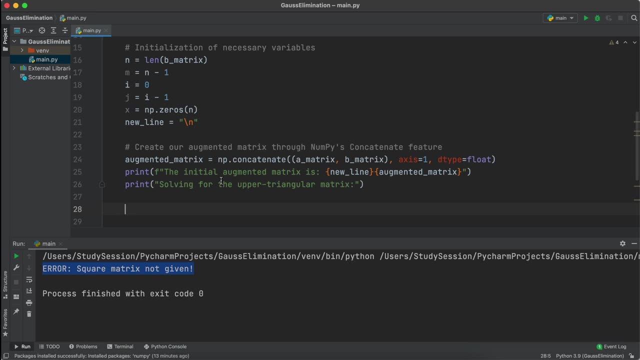 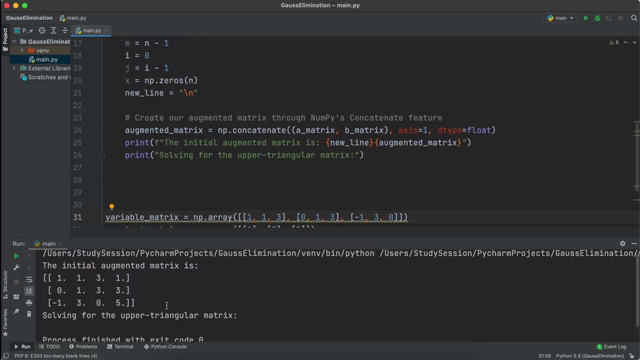 matrix and that shows that we are now beginning to solve the matrix using Gauss elimination. And, although a bit unnecessary, I like visualizing my code like this and, if you are like me, it allows for a more proper understanding of the code and helps us to identify if there are any errors occurring. 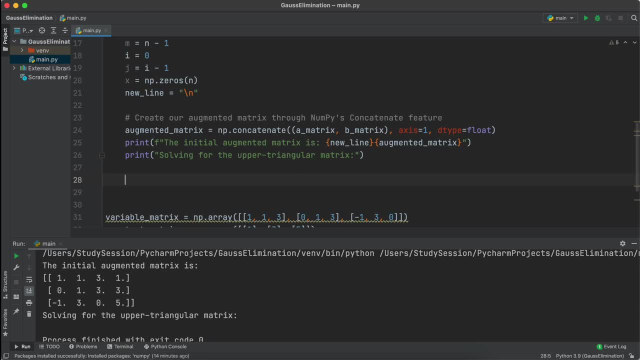 Now our Gauss elimination will be completed under this while loop. We say that while i, which is an iterating variable, Is less than n- our number of rows, We run the code within the while loop. Firstly, if you have a zero on our main diagonal, we are going to run into issues with our scaling. 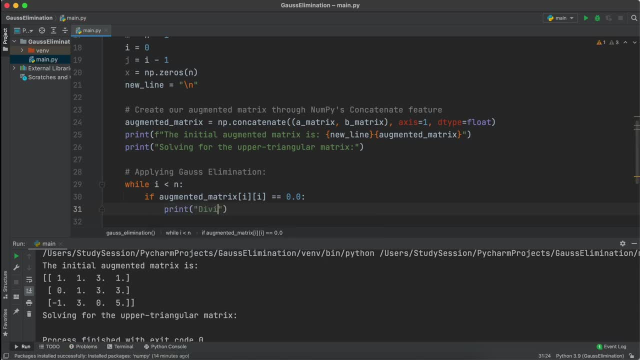 factor formula. Therefore, let's add a print error in return, like we did previously. In a future video I will make a gauss elimination function that also actively does partial pivoting. When complete, I will add that video to the description down below. 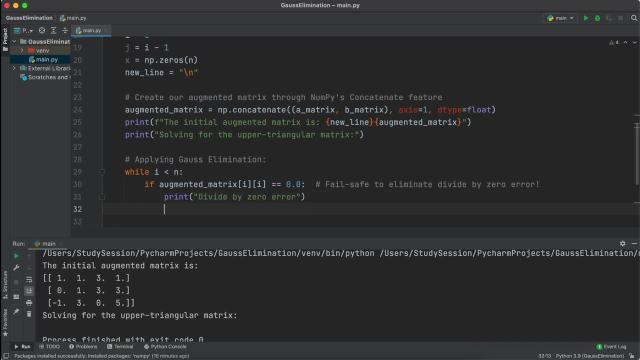 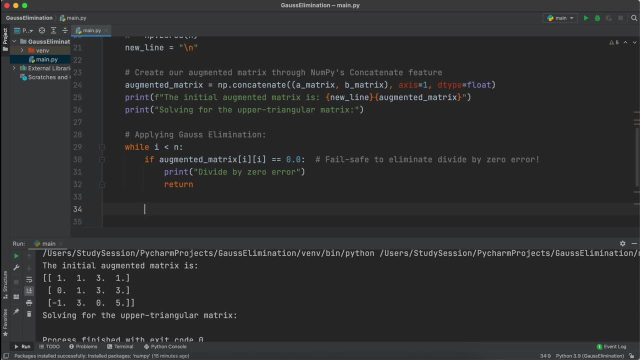 So check there if you are looking to add partial pivoting to your gauss elimination function. However, for now, assuming we have no zeros on the diagonals, let's begin going row by row and systematically convert all of our elements below the main diagonal to zero. 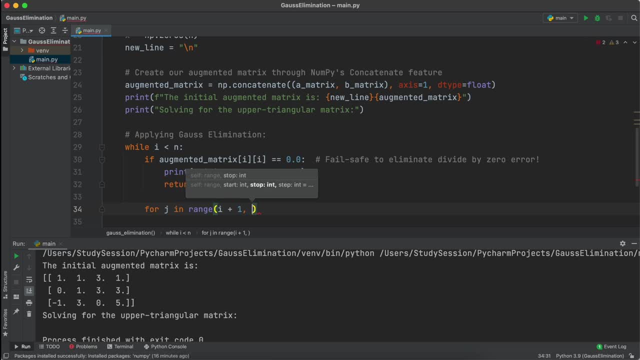 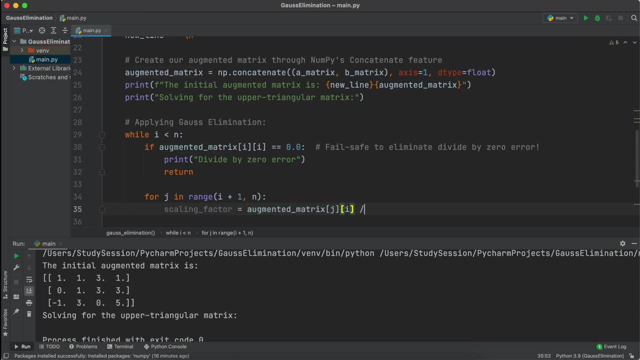 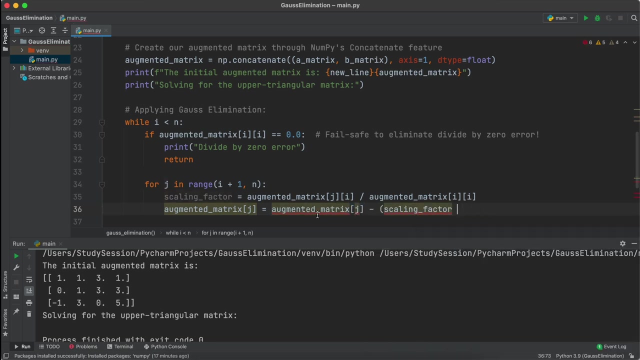 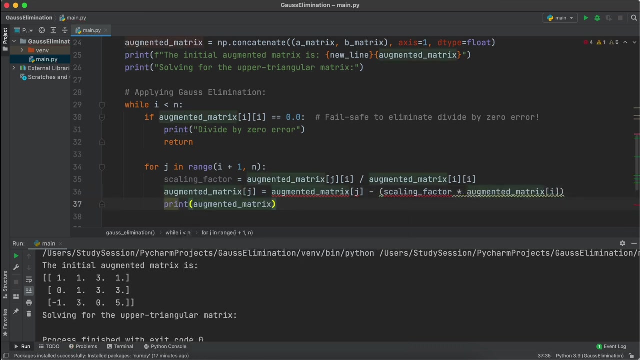 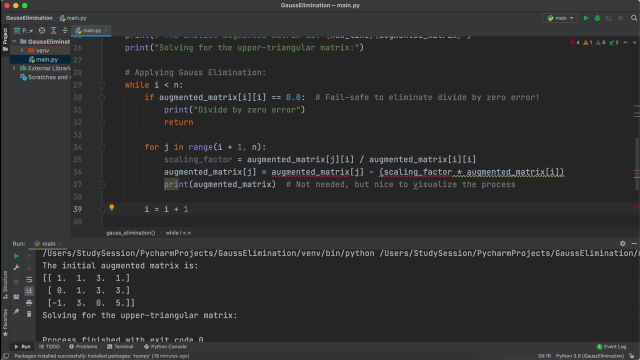 So this: if statement is saying: while our iterating variable j, which is currently i plus 1, up to our number of rows n, complete the row by row reductions, Then we need to increase our iteration counter i And then we are done the gauss elimination row augmentation. 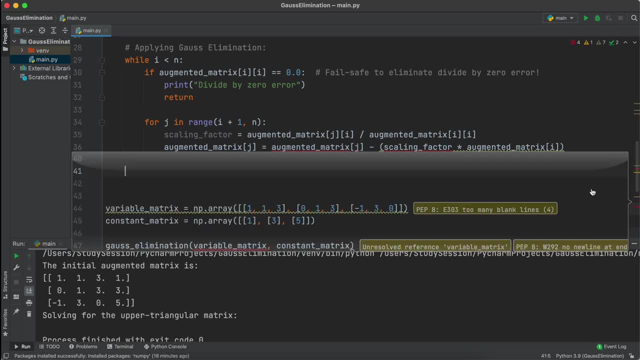 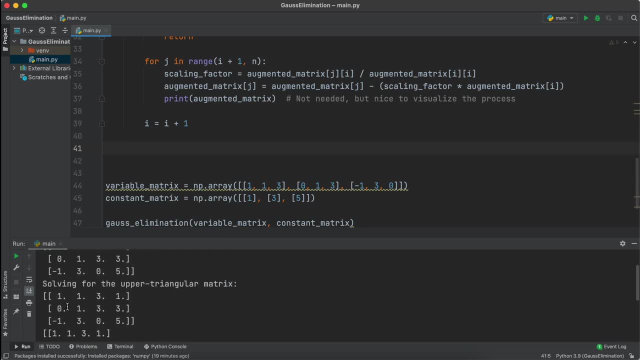 So at this point it would be logical to test our system using some matrices. So let's do that now And, As you can see, we reduce our column 1 row by row first, And then we move on to the next column, but moving down our main diagonal with each increase. 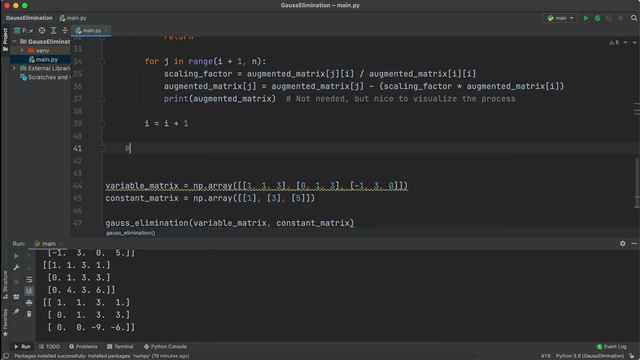 of i. Our final step of gauss elimination is we need to complete backwards substitution, starting with our last row of our augmented matrix and working our way up. We begin by initializing our backwards substitution by solving for our first x value, So we only need to divide our bottom right most element. 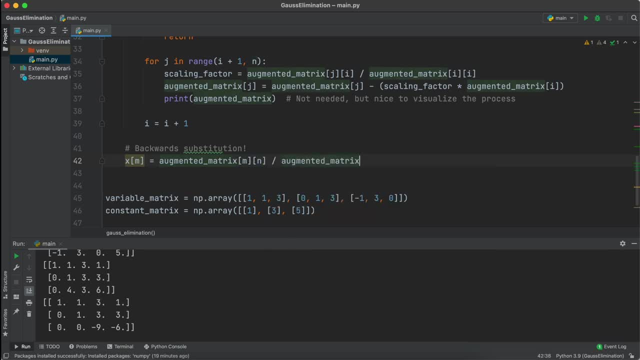 So m rows And n columns. Since our augmented matrix is always going to be one column longer By our xm value at the bottom of our matrix, This solves for the bottom value of our x matrix. Lastly, let's begin the backwards substitution algorithm, which works by beginning at our 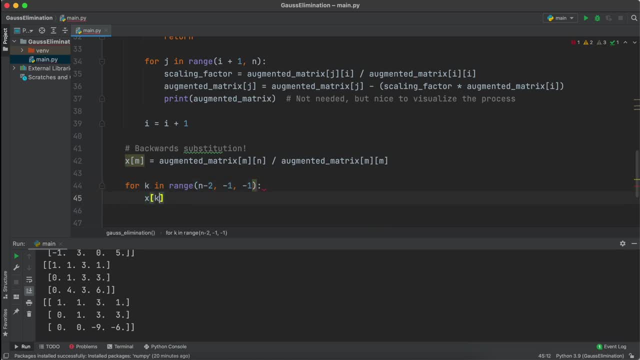 second last row, since we have just previously solved the bottom row. This range function will begin at n-2, so our second last row And We need to complete the rows by taking minus 1 steps, meaning that we are climbing up our 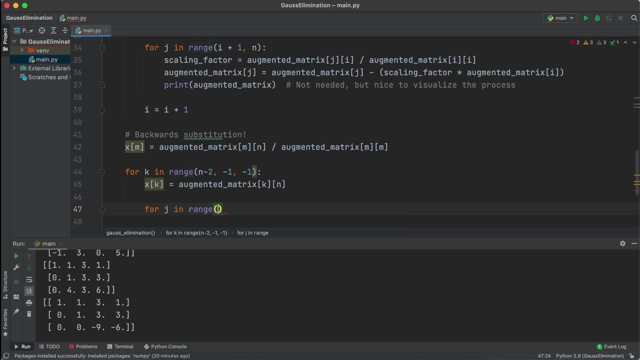 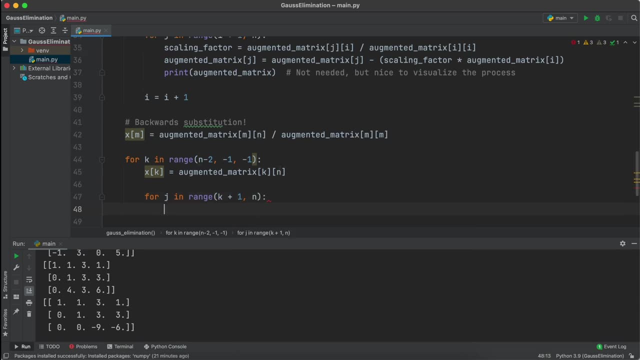 matrix, with each iteration up to minus 1, as the range does not include, to the end step. So a zero here will ignore our first or top row, So you need minus 1 as your end step. Lastly, this line here will go through and complete all the relevant element by element. 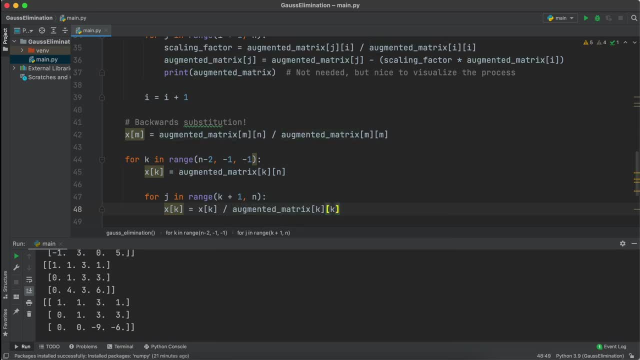 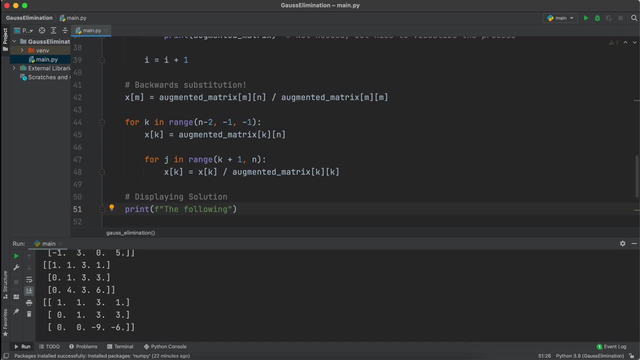 algebra and add it to our x vector matrix. Lastly, let's display the results to our user. To do so, I'm going to do it in a for loop like so, as I think it looks nice, I will save for temporary variable answer within our range of n and in this first curly.